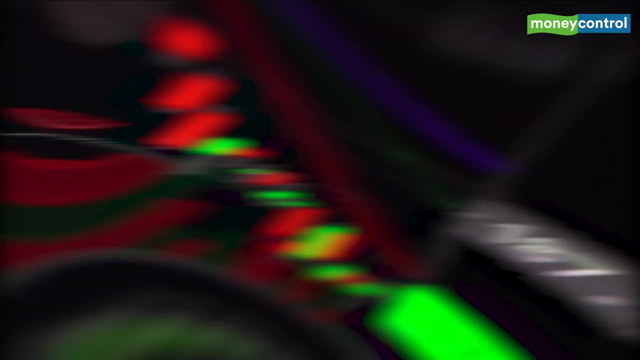 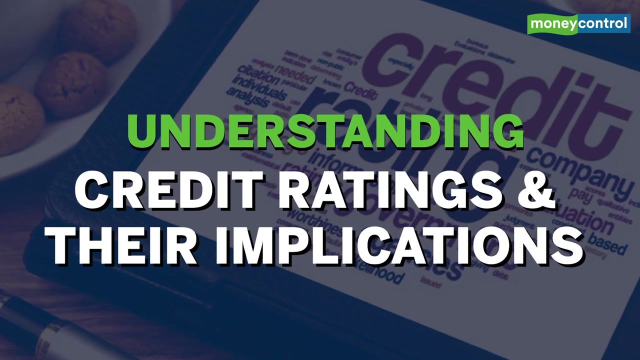 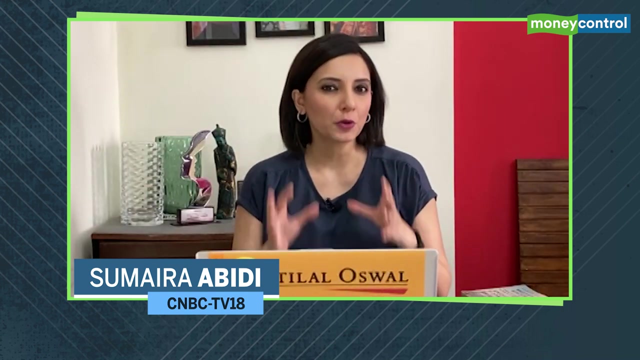 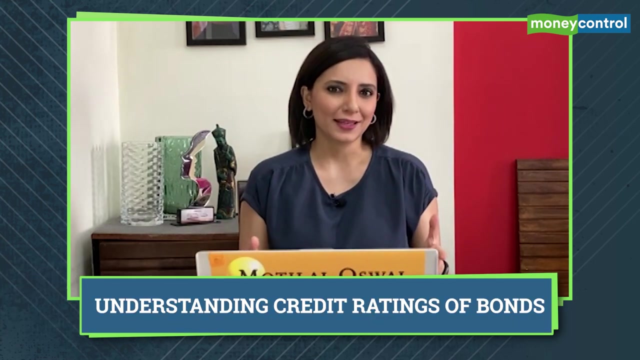 The focus of the retail investor in debt mutual funds has really now shifted to the credit quality of the bonds in those portfolios, And this is measured using the credit rating. So credit rating is nothing. It's just a score which evaluates the quality of the company and judges. 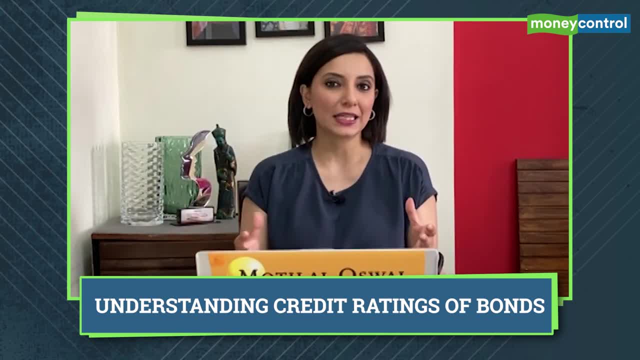 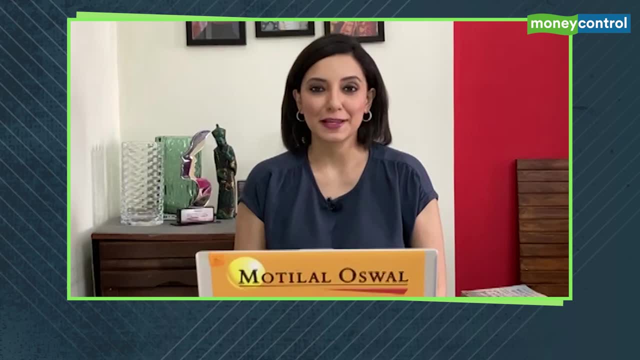 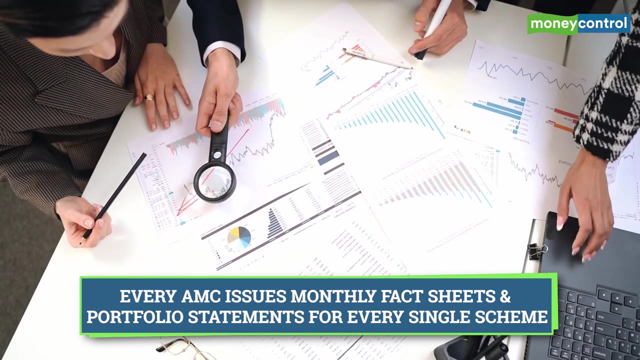 them in respect of their ability to repay the money on time. So today, let's take a look at what credit ratings of bonds are and how you can understand them correctly. Every AMC will issue monthly fact sheets and portfolio statements for every single scheme, Among many other important 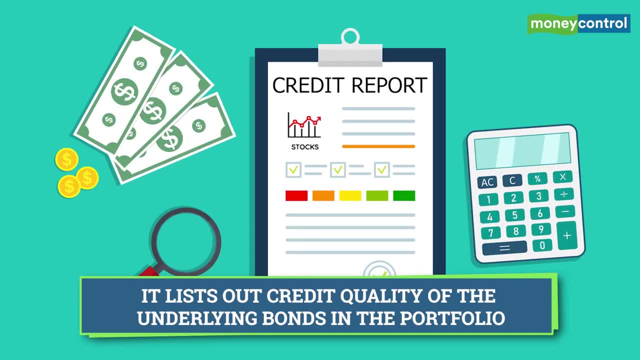 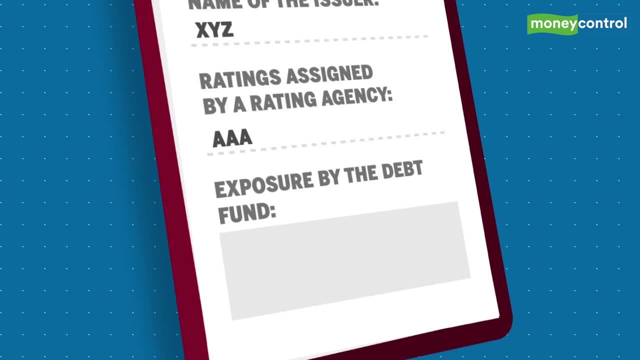 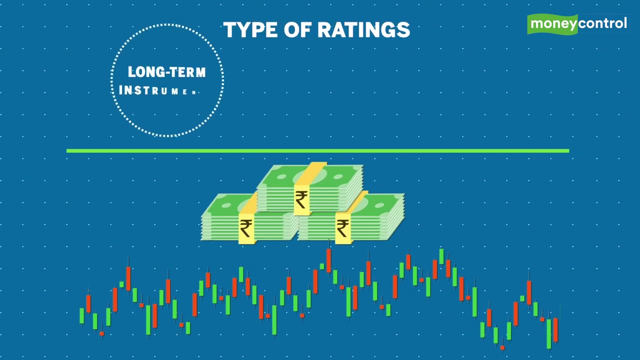 things. this statement lists out the credit quality of the underlying bonds. in the portfolio One can find the name of the issuer, the rating assigned by a rating agency and the exposure by the debt fund. Primarily, there are two types of ratings: one for long-term instruments and one. 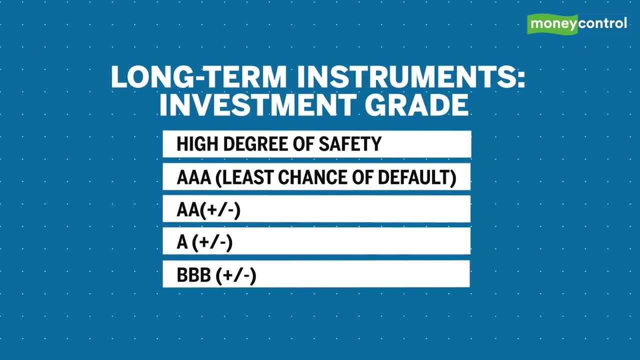 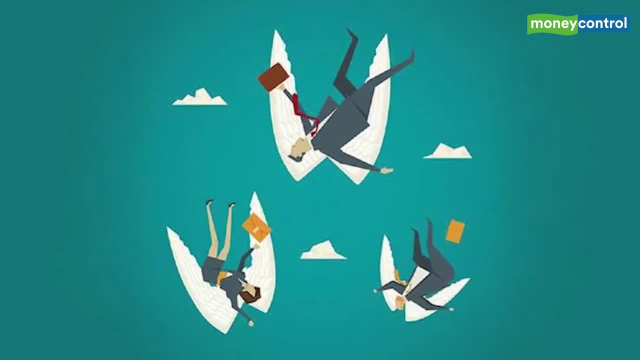 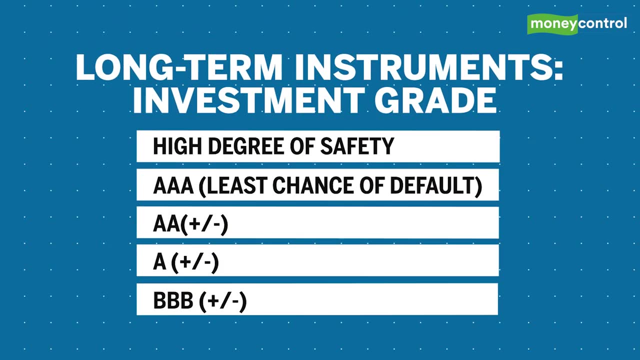 for short-term instruments. Within long-term, the highest notch is AAA, which means it has the least chance of default. Do note that this does not mean cannot default. It just means it has the lowest probability. The investment grade ratings continue downwards all the way to BBB plus or 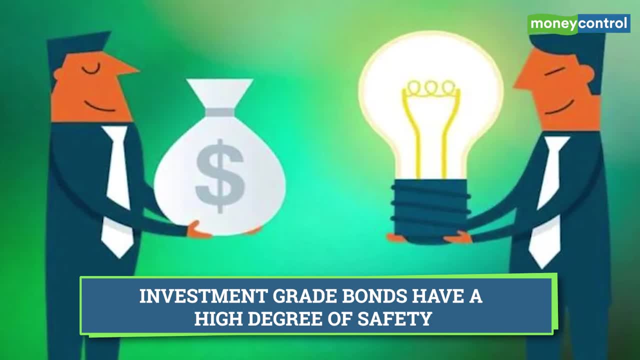 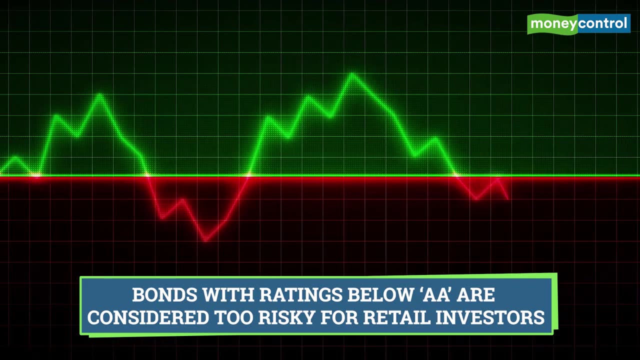 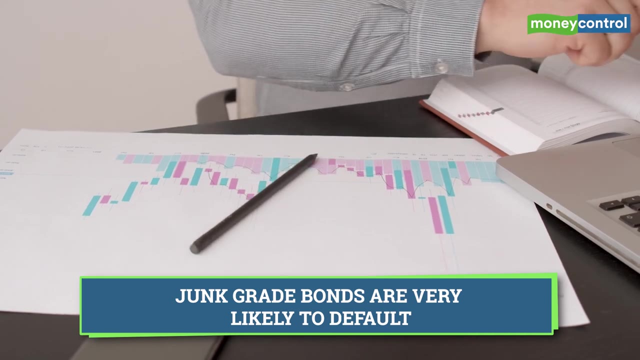 minus The investment grade set of bonds are said to have a high degree of safety. But even within this bracket, bonds with ratings below AA are considered too risky for retail investors, And there are bonds which are considered below investment grade or junk grade, which are 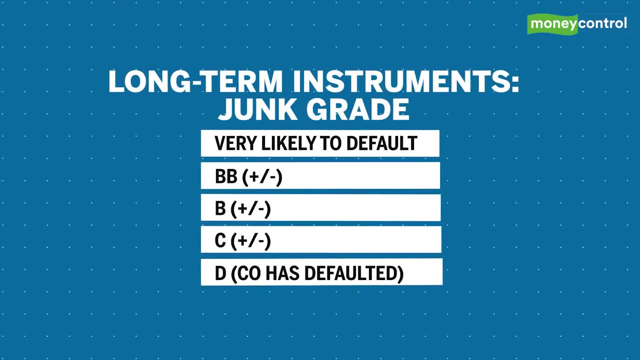 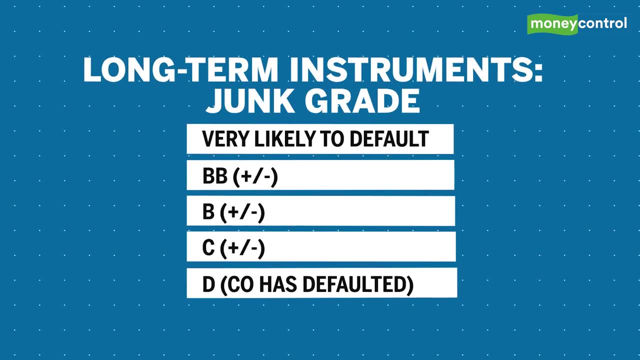 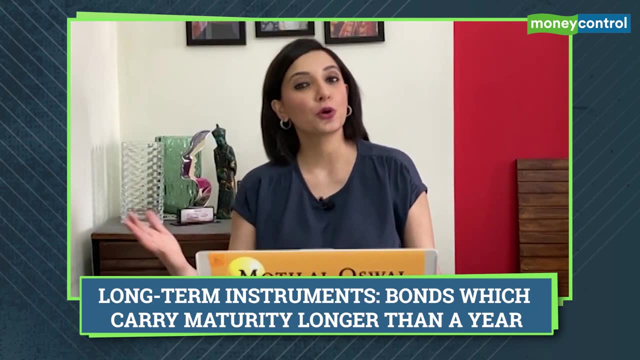 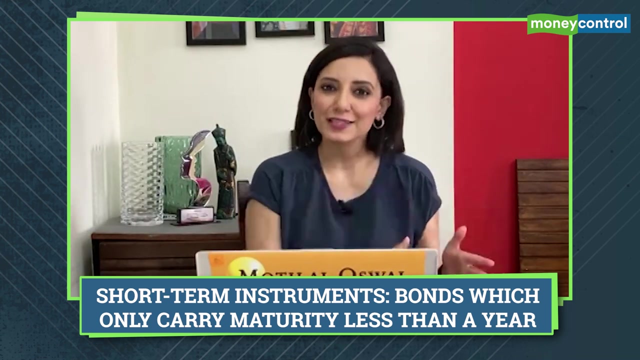 considered to be very likely candidates to default. This list starts from BBB plus or minus and ends at D, which means a default has taken place. Long-term essentially means that the bond will have a tenure or maturity which is longer than one year. Conversely, short-term will mean bonds which have a maturity or tenure of less than one.